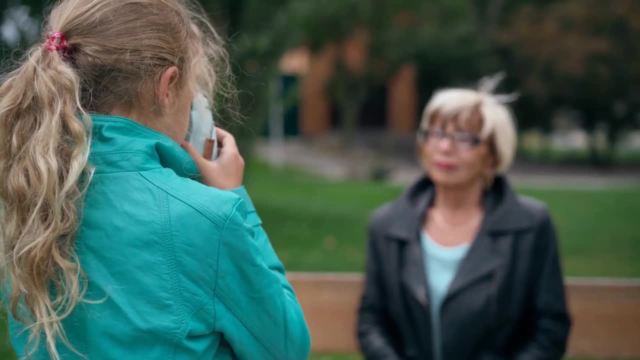 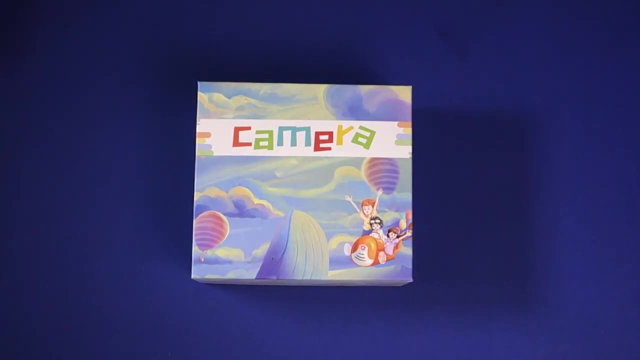 cameras for my 11 and 6 year olds so they can have fun documenting their own vacation experience while keeping them occupied. In this video, I take a look at two very fun, inexpensive digital cameras: the Bofipu vlogging camera and the Tondozen kids camera. 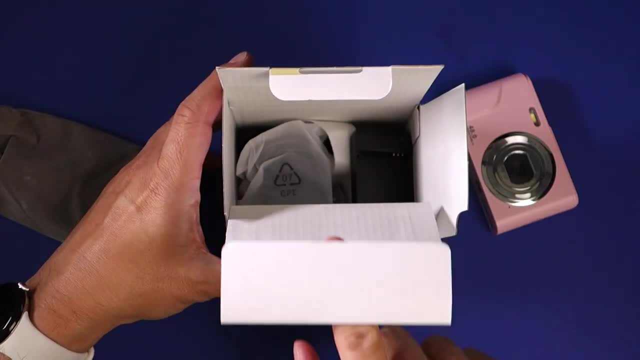 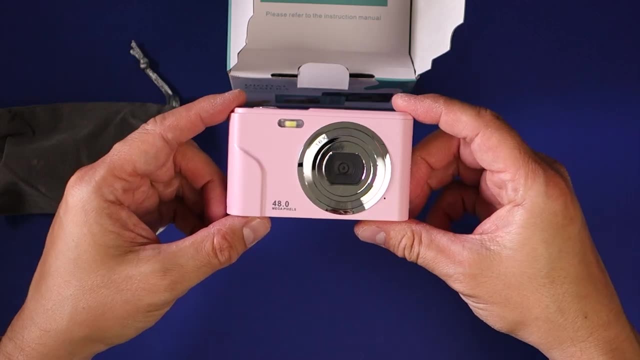 When it comes to the Bofipu vlogging camera, it's actually pretty well stocked for content and accessories. The camera itself is made of a plastic and very lightweight, which you'd expect for the $112 price tag. However, the silver buttons all appear to be metal, which will hopefully help with durability. The 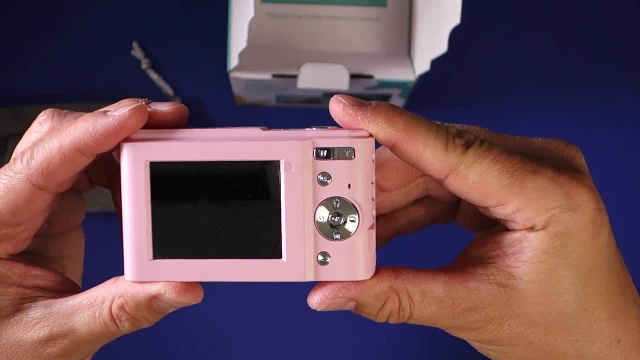 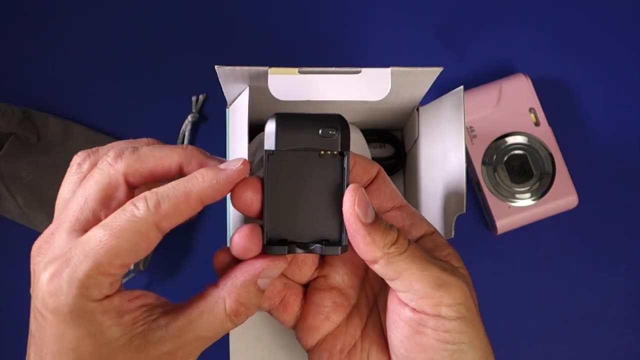 design actually reminds me of one of my first ever Sony cameras from 20 years ago. The layout is very familiar. While you can charge the battery in the camera, it's packaged with a small battery cradle that you can use to connect to a power supply, with the included USB-A to mini USB cable. and there's a good reason. 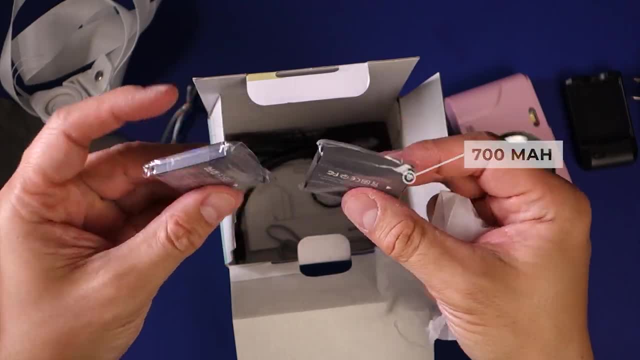 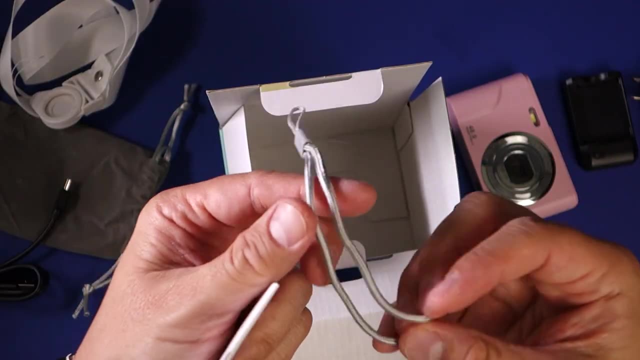 for the extra hardware, as the camera comes with a second battery. Other accessories include the power brick and two different straps, One with a quick release that goes around your neck, and the other is a wrist strap. What the camera doesn't include is a memory card, but thankfully there are some. 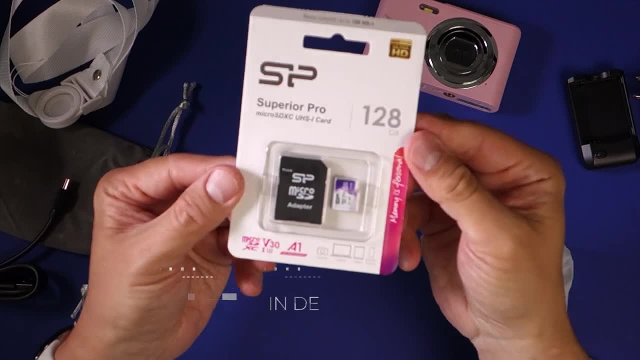 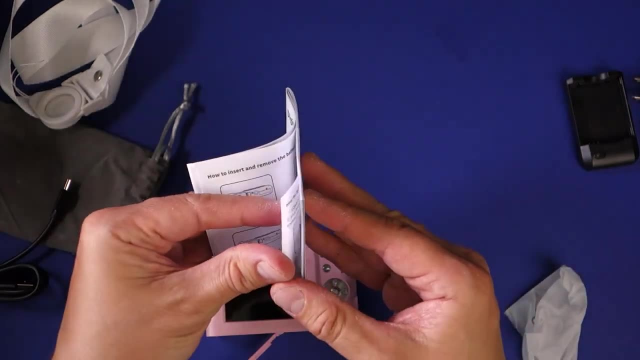 inexpensive options on average. I decided to try my luck with the silicon power 128 gigabytes micro SD card, and I bought it for only $13 on sale. but Bofipu doesn't recommend using U3 class memory cards, so we'll see if I end up having to buy something more. 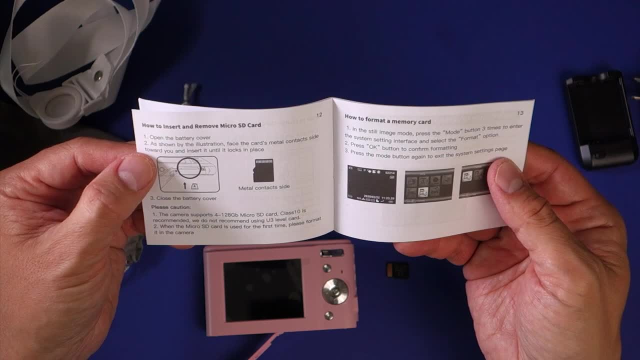 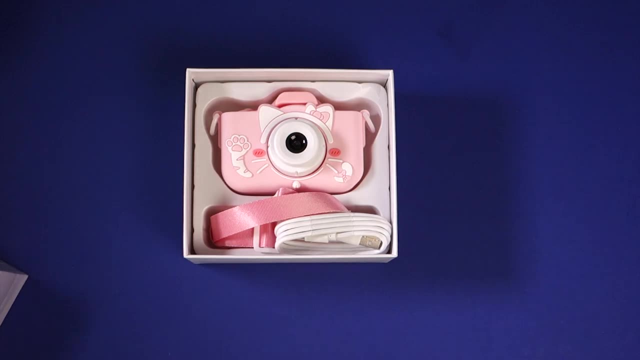 expensive later. Through my early testing, though, it worked fine. The Tondozen kids camera has fewer accessories, but that's expected for the much lower price point. Inside the Tondozen box you'll find the camera itself, which is already in its very fun silicon-powered box. 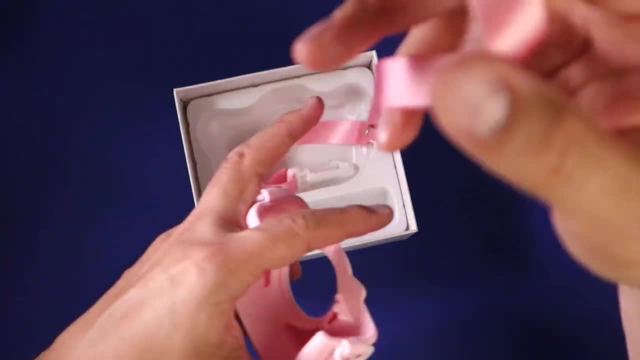 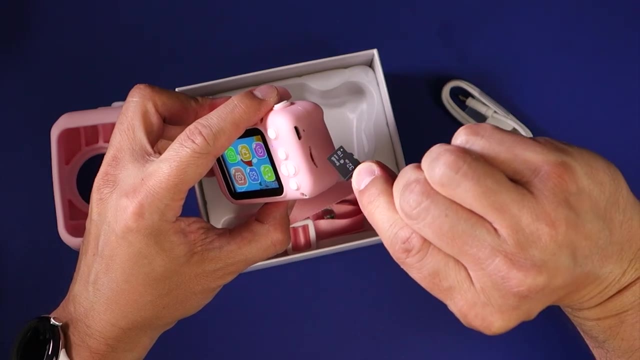 Plus there's a charging cable and there's a nice neck strap. One nice touch is that the Tondozen kids camera does come with a 32 gigabyte u3 memory card, which saves owners a bit of money. The camera does support up to 128 gigabytes. 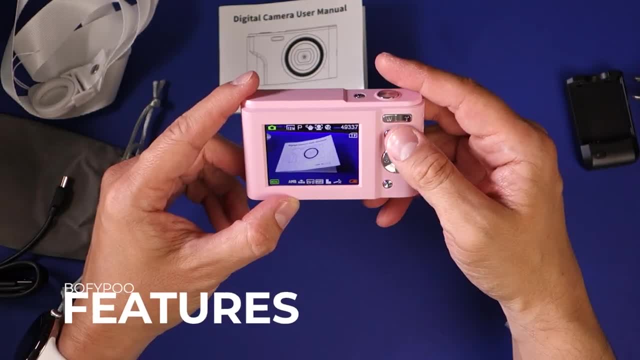 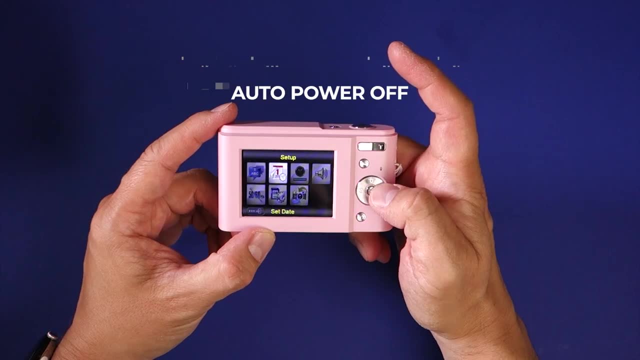 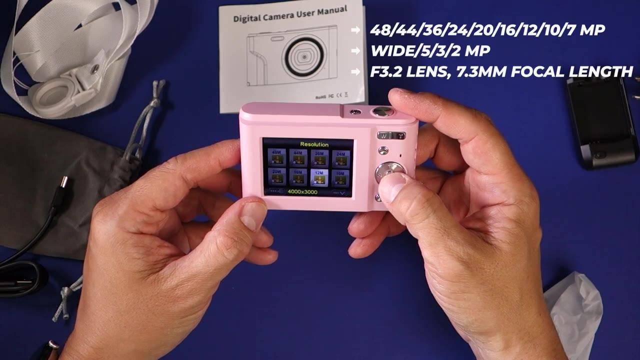 if you do want to upgrade, though, The Bofipu camera has a bunch of pretty standard features, including a 16 times digital zoom and an auto power off mode, which is actually ideal for forgetful children to make sure that the camera has power when they actually need it. In terms of the photography options, 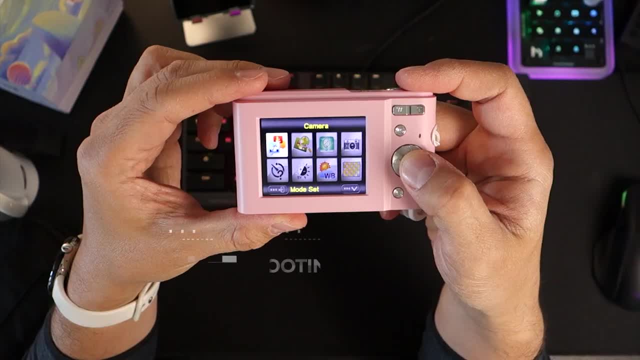 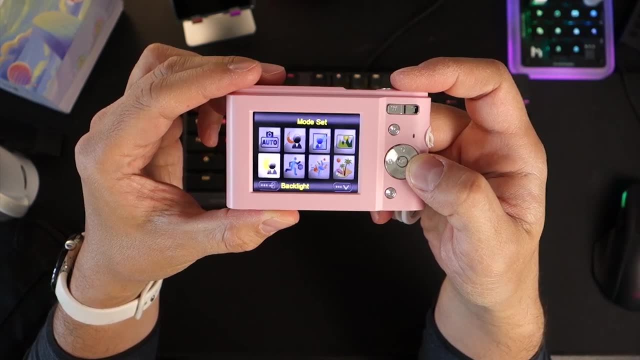 it includes a lot of different resolutions for such a cheap camera Plus, there are nine different shooting modes to choose from, including the default auto option. While it's nice to have the options, I'm fairly certain my 11 year old will keep it in auto mode most of the time. When set to auto the camera 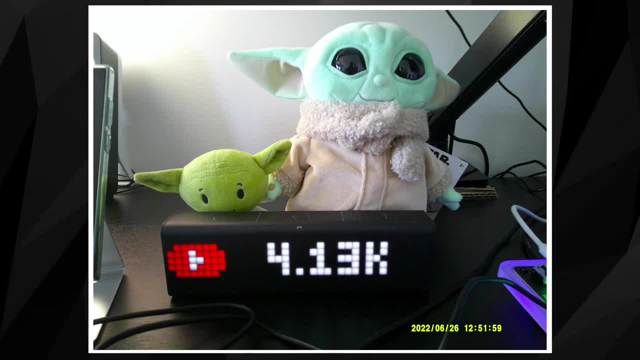 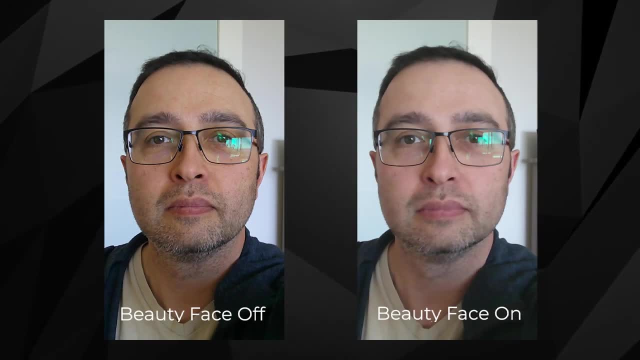 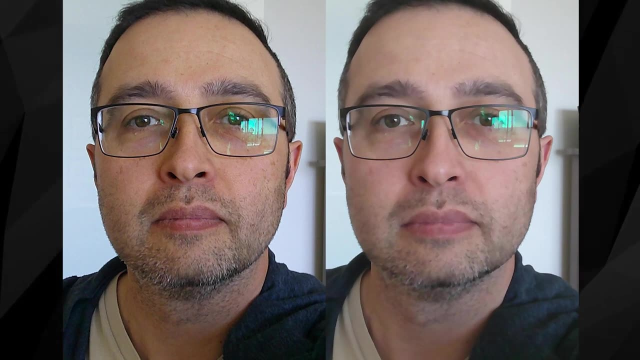 will automatically choose the best settings based on the subject, lighting and composition. One additional fun feature is beauty face, which digitally touches up any portrait images. It's a feature that's widely available in more expensive digital cameras and also mobile phones. now The feature applies an artificial cosmetic look that smooths 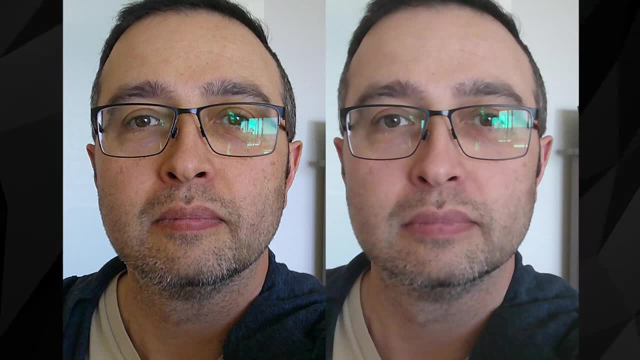 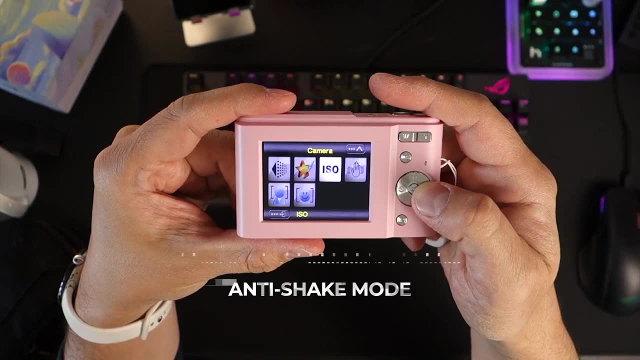 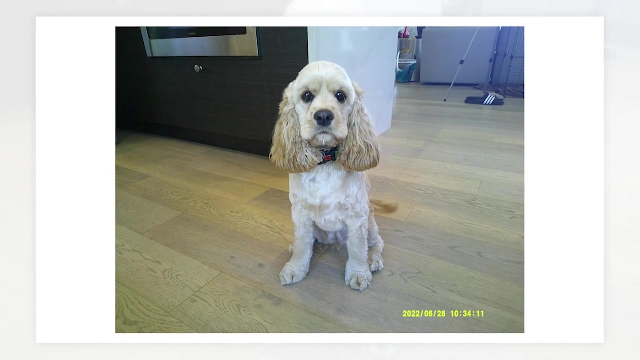 out the skin of a subject to appear more appealing. The camera also features a self timer for taking selfies, with or without a tripod. The final main feature is the anti shake mode that applies some digital stabilization to keep photos in focus. Checking the images, I was expecting it to crop the image to. 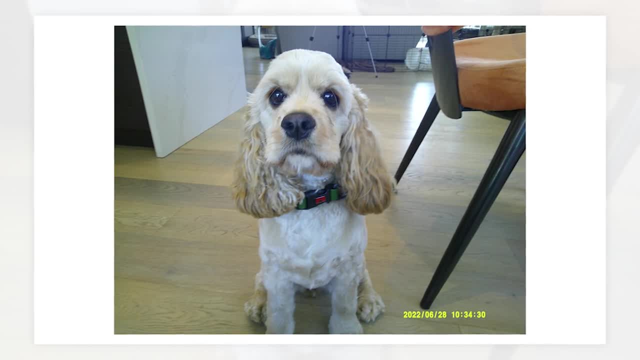 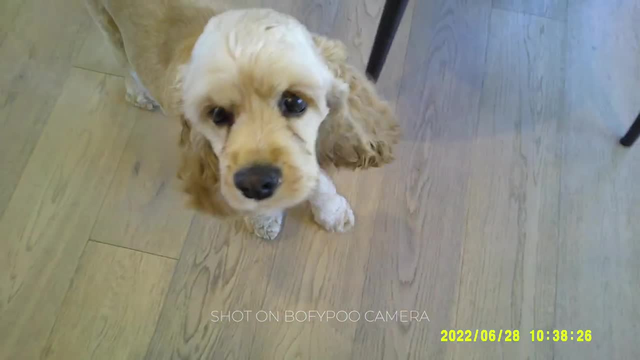 achieve the effect, but I couldn't really detect any changes that would adversely affect the images. The options for videography are much more limited. as far as I can tell, There is just the option to swap between 1080p, 720p or 480p. 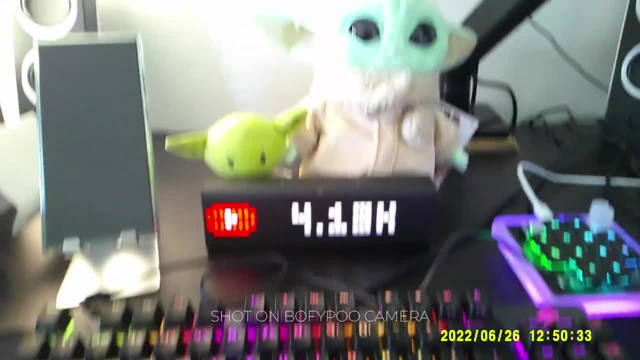 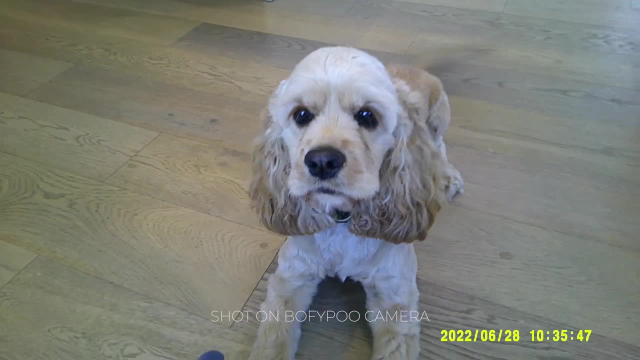 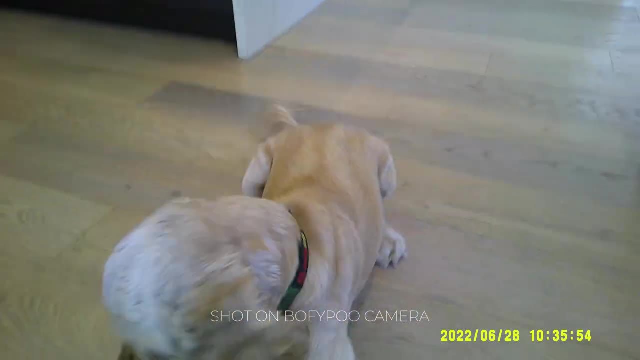 resolution. My own inclination and recommendation is to leave the camera in 1080p. Most modern devices you'd use to review the content, such as modern TVs, computers and phones, start at 1080p resolution and are usually much higher resolution, Provided you have a big enough memory card installed shooting. 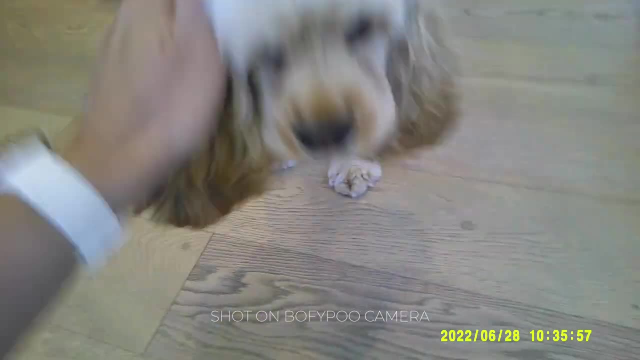 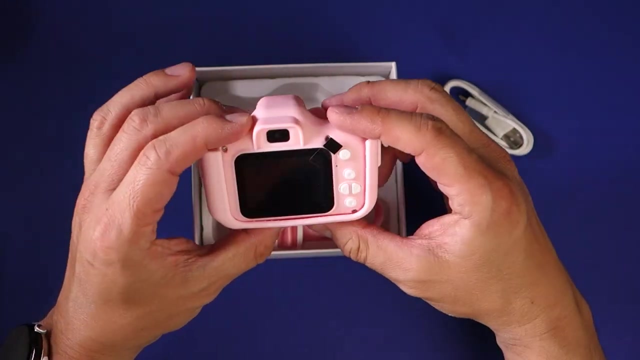 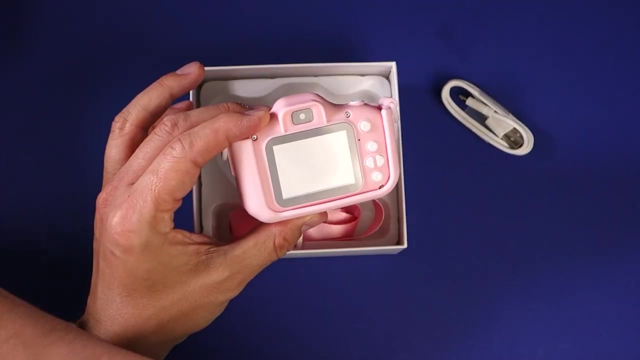 everything in the higher resolution won't really affect your ability to store lots of videos. The Tondozen, by comparison to this surprisingly impressive Bofipoo camera, is very much positioned as a toy. The design, build and performance for photographs and videos are all acceptable. for the $33 I paid on sale, The photographs captured a low. 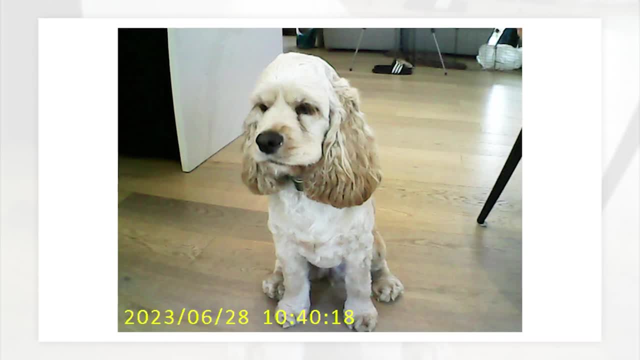 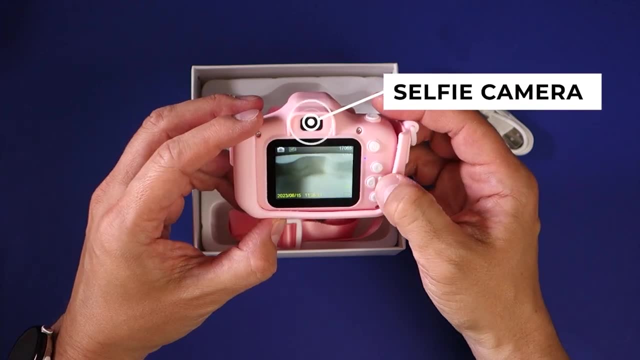 resolution and reflect the quality of a cheap lens and sensor, even though it captures a maximum of 12 megapixel images. There is a fun selfie mode using a tiny camera on the reverse, where the fake viewfinder is located. Just like the still images, the video performance is.